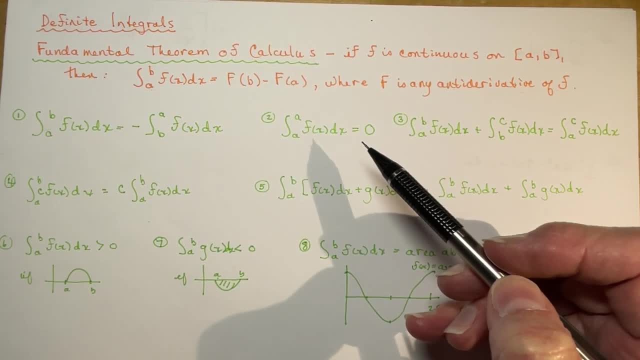 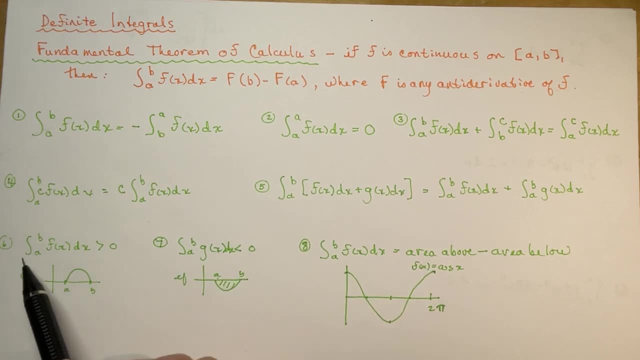 because it's just going to be plus c, minus c, so no c. Okay, so let's look at a few of the rules. They're very straightforward and easy to understand. I believe It says that if you have a definite integral evaluated between a and b of f at x, dx. 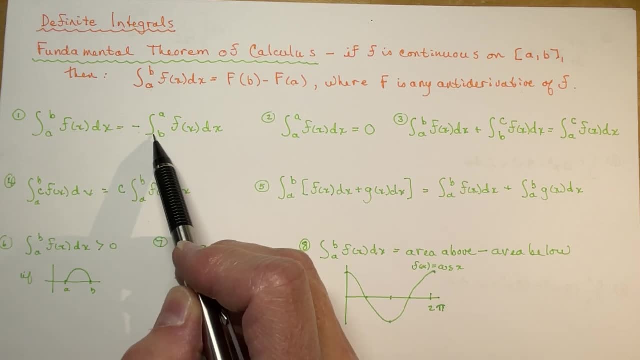 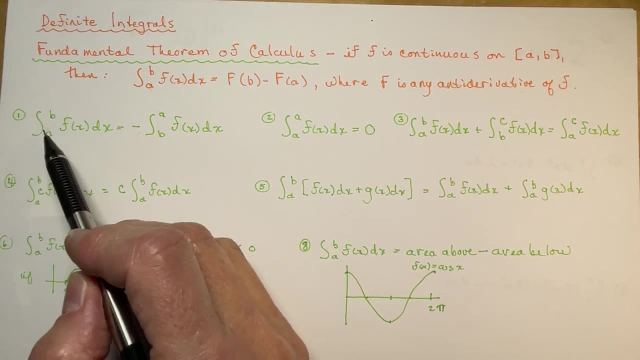 that's equal to the negative of the integral from a to b, so a to b or b to a. So if I do it backwards, in other words when I go to evaluate this, I would do f at b minus f at a. 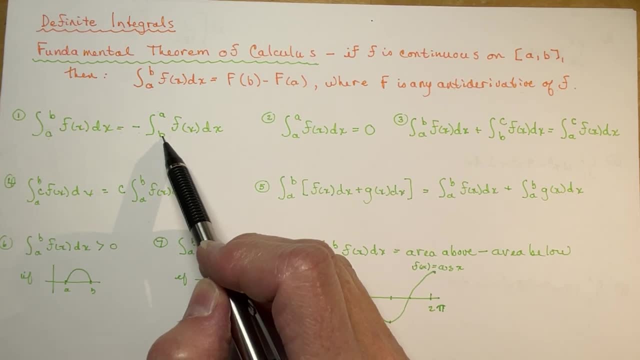 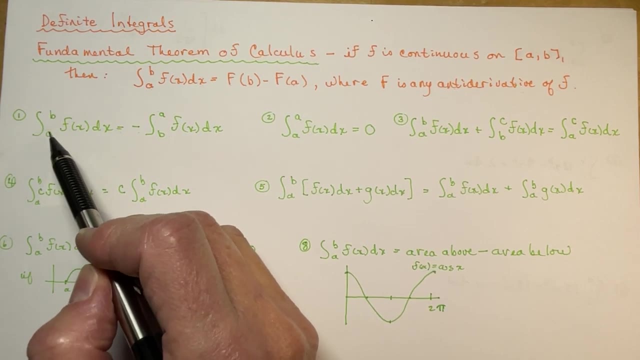 And this time I'm doing f at a minus f at b. So you can see, if I had, if this was 5 and this was 1, I would have. 5 minus 1 would give me 4.. And if I had 1 and 5 here, 1 minus 5 would be minus 4.. 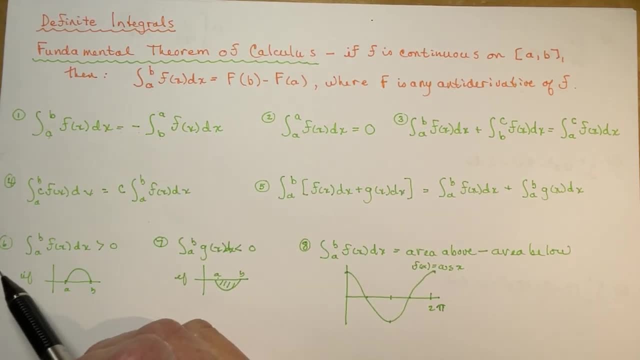 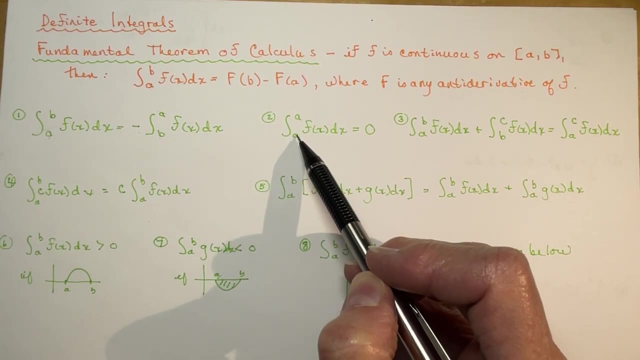 So the minus of that is equal to this one. That's all that one says. Example 2 here says: if I have a definite integral that has the same boundary, so a to a, that means the area is going to be 0.. 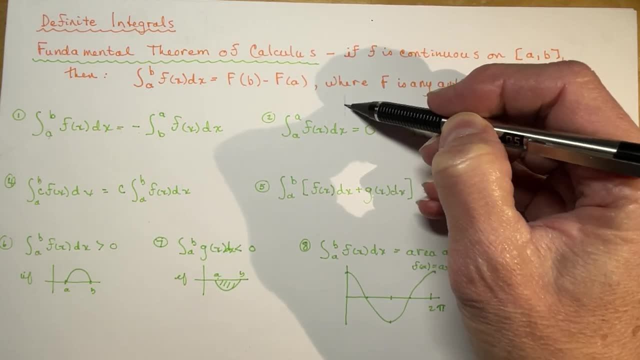 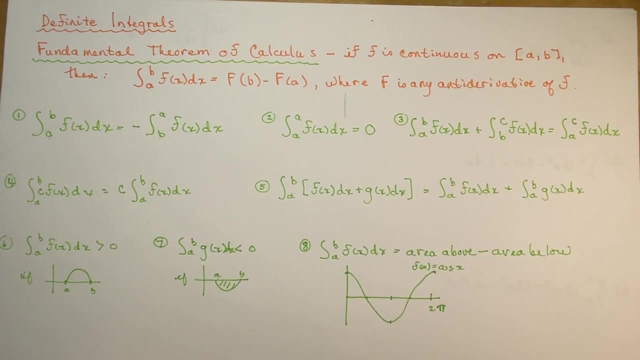 Because basically you're talking about the area under a point, So a straight line. basically There's no area to it, So that's why it says that the area is equal to 0.. Now if I have a definite integral from a to b, of f at x, dx. 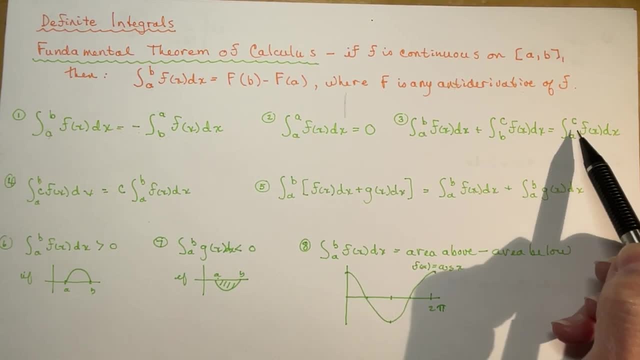 and from b to c, of f at x, dx. that's the same as evaluating it from a to c. In other words, all you're doing is you're just adding, adding the two areas together, so you might as well evaluate them all at once. 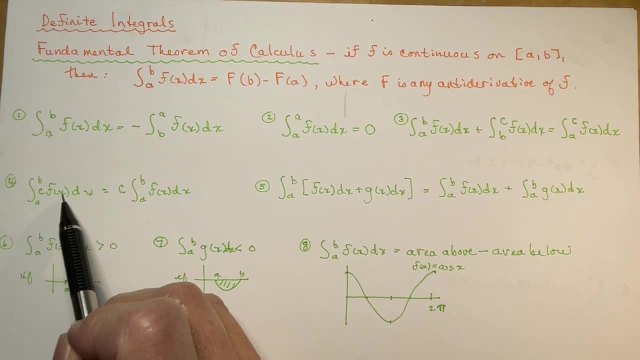 Now if you have a constant times a function and you're taking the definite integral of that, that c is actually with this part here, then I can take the constant out front and evaluate the integral between a and b. Pretty basic right. 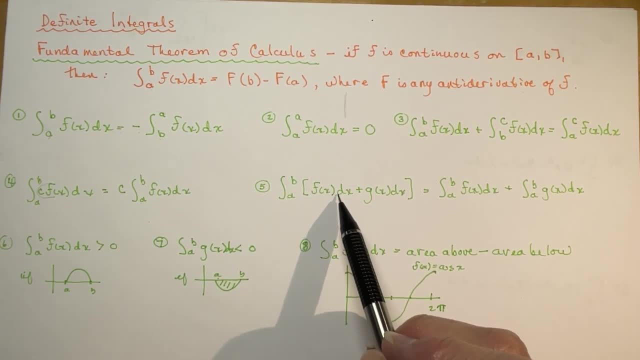 And similarly, if I have something like f at x dx plus g at x dx, I can evaluate them separately and add them together. Now also, if my integral, my function, is above the x axis, then this area is going to be greater than 0.. 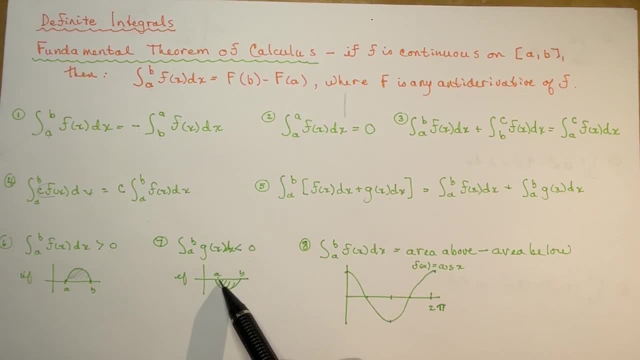 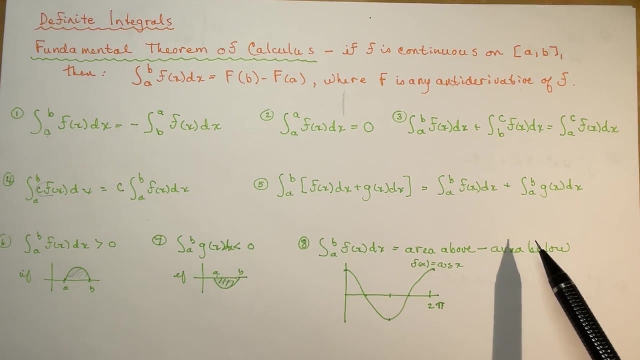 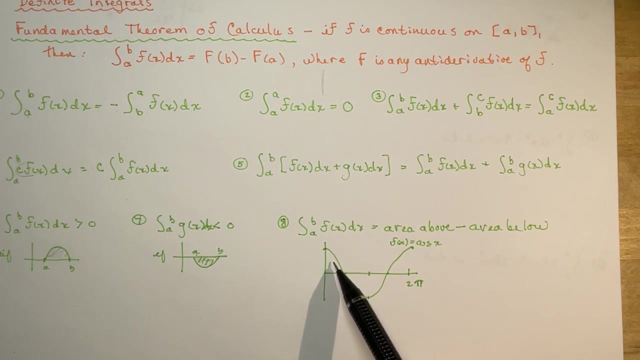 But if my function is underneath the x axis, then this area is going to be negative. Now if I had a function where I'm going between a and b and some of it has area above and some of it is below, For instance, if I had the function 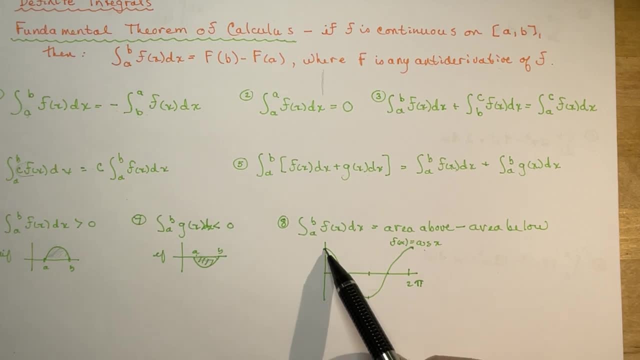 cos x and I evaluated the area between here and here, so let's say between zero and two pi. if I evaluate that, then I'm going to end up with an area of zero. Let's just try that for a second and I'll explain how that all works. So I want to know what is the integral between zero and two pi? 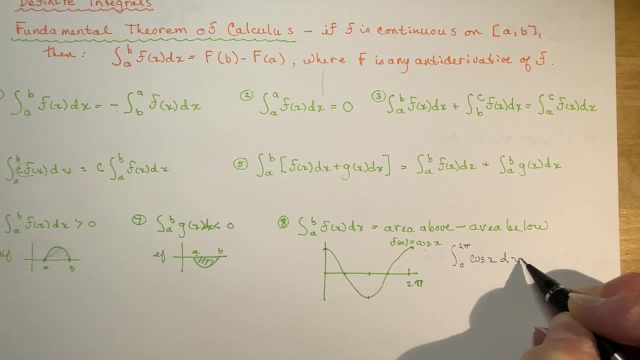 of the cos of x- dx. There's my cos Starts at one minus one zero to two. pi is the period. So the integral or the antideriv of cos x, of course, is sine x. so I'm going to be evaluating sine x between zero and two pi. 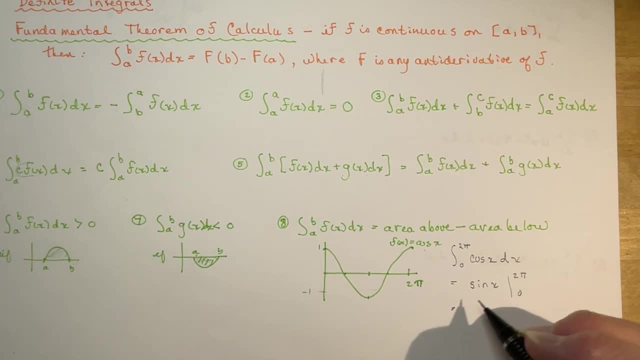 So that means I'm going to do the sine of two pi minus the sine of zero and if you recall your sine function, quick sketch, that's zero and zero and I get zero. So I'm going to get zero area. and again, that's because this part and this part added together is the same as this part. 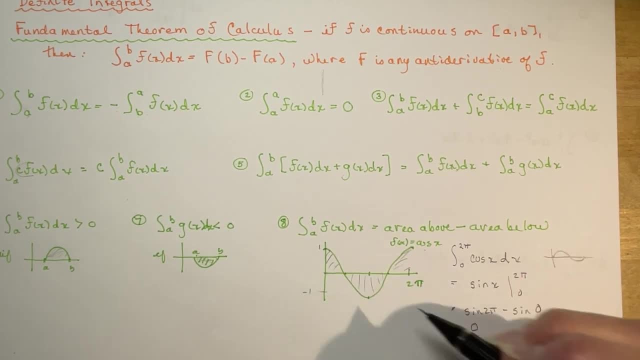 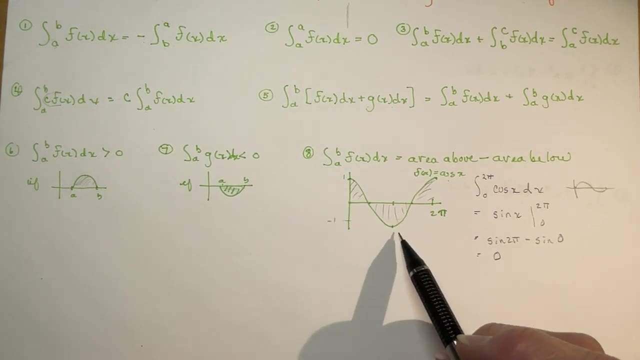 but this part is all under. So this is positive, this is negative and this is negative. So I'm going to do the sine and this is negative and I'm subtracting them away from each other. So if you were to look at this and try to find a part that would give you a positive or negative. 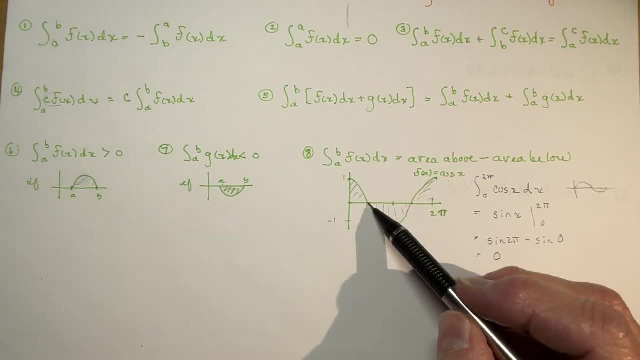 area you'd have to look at either between zero and remember: this is pi, this is pi over two. So I asked you, if I asked you between zero and pi over two, you would get a positive area. If I asked you between zero and two pi, then you would get. 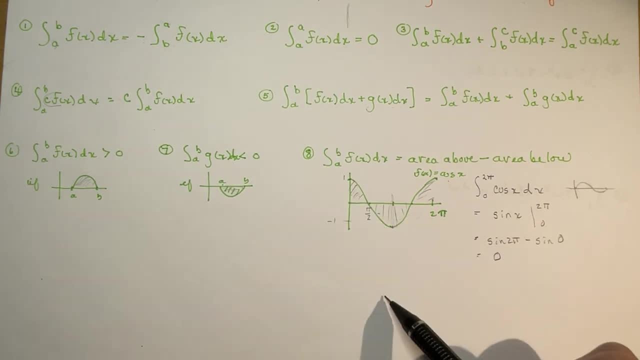 zero again, because these two would cancel out. If I did between pi, pi over two and three pi over two, then I would get this negative area down here and you can try those if you want. Well, let's just do one of them. Let's say what if I did the integral between zero and pi over two? So I just want this. 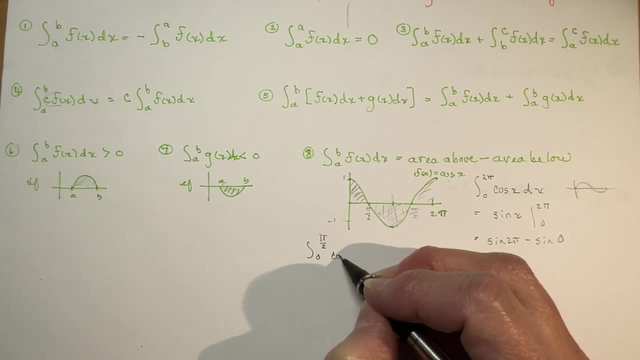 part right here of cos x, dx, That's going to be equal to the sine of x between zero and pi over two, and that would give me the sine of pi over two minus the sine of zero and the sine of pi over two. Remember that was one. 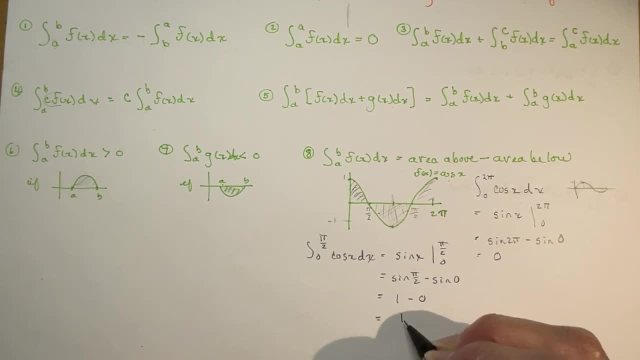 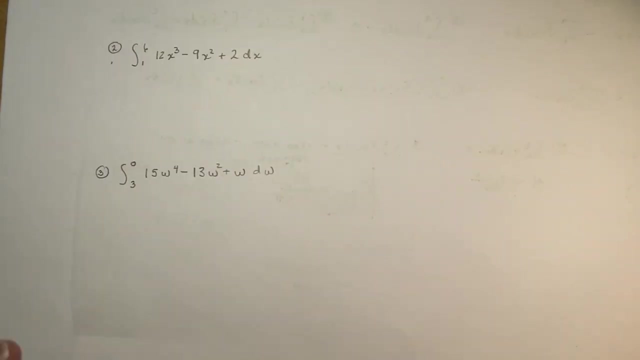 so I have one minus zero, so I would get one, Okay, so basically, those are the, the rules that you might have to work with, which gives you a little bit of flexibility in your calculations. Okay, so let's go to some examples. first, Let's find what is the definite integral between zero. 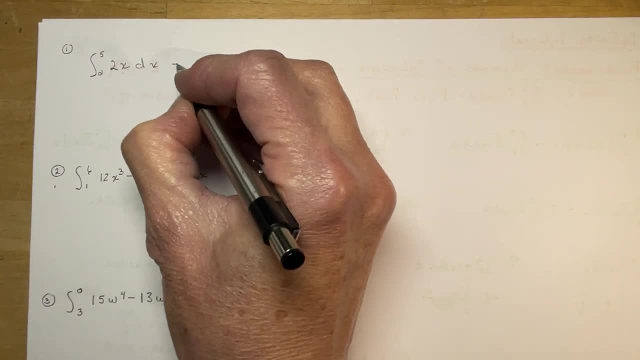 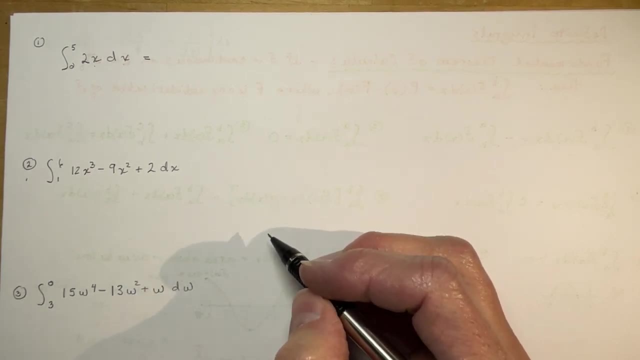 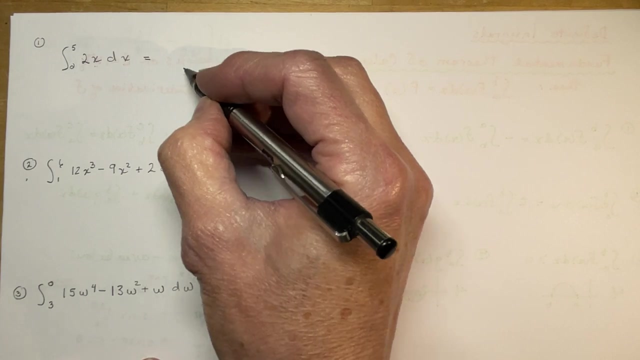 and five of two x dx. Now don't forget your equal signs. I noticed in some of the other videos and some places people forget those and and that's important when you're doing this. So let's go to some examples. So if I want to know what the antiderivative of two x is, I would add one to the exponent, that's two. 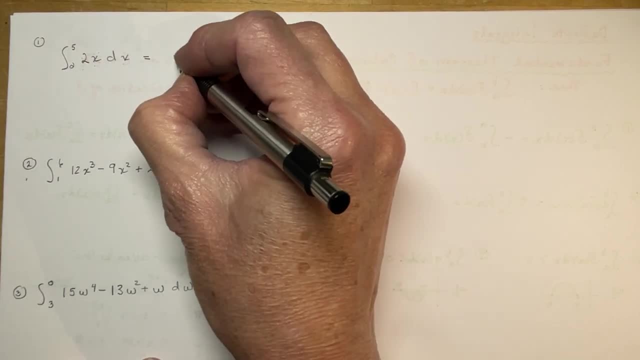 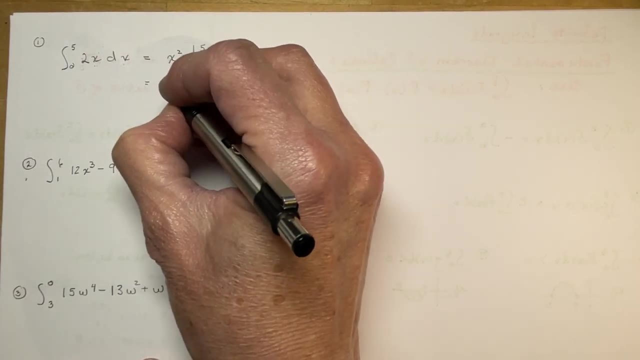 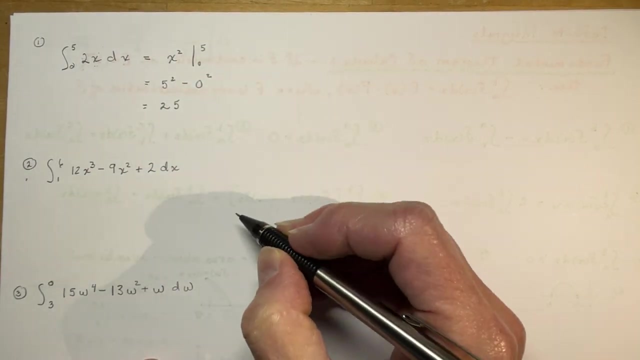 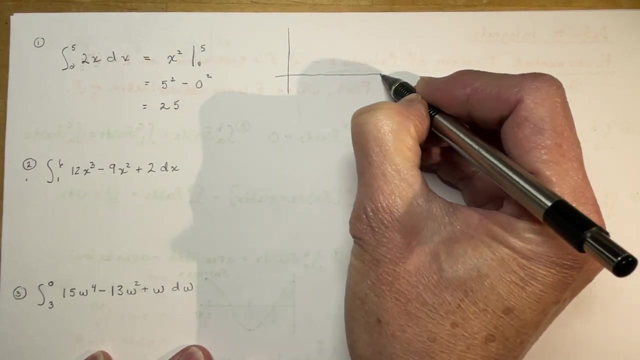 divided by two. so I get x squared right. so x squared between zero and five. So that's going to be five squared minus zero squared equals 25.. Now if you think about this, and let's just make a quick little sketch of what this actually looks like, the line 2x between zero and five. 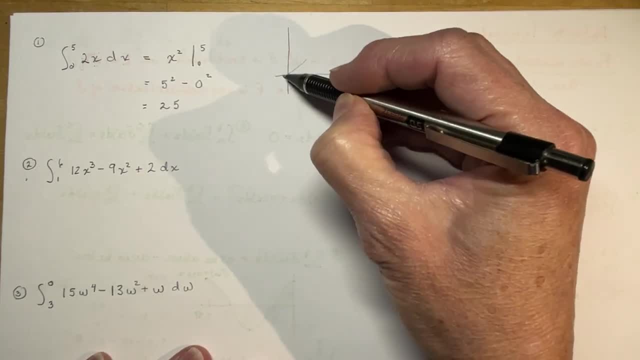 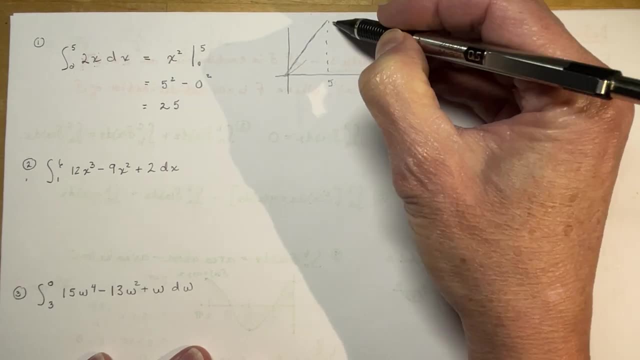 that's going to be twice the steepness. that would be like an x at 45 degrees. so it's going to be kind of very wiggly line. so if I went to five, the height of this triangle, when x is five, y would be two times five or ten. so I would have 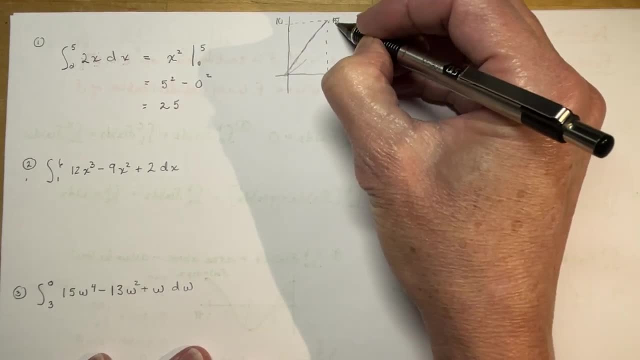 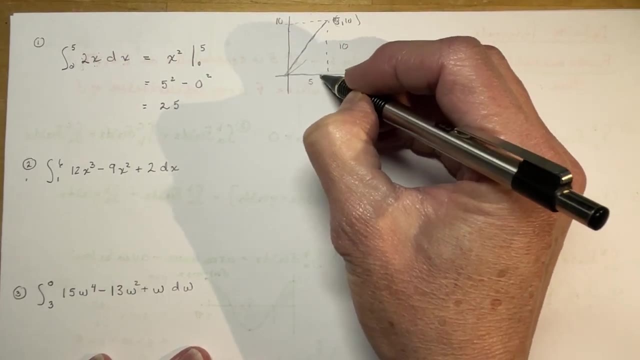 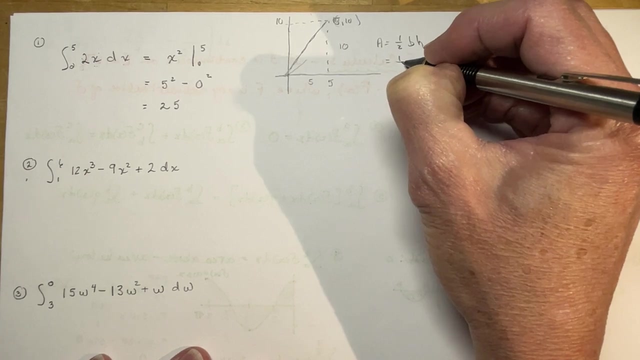 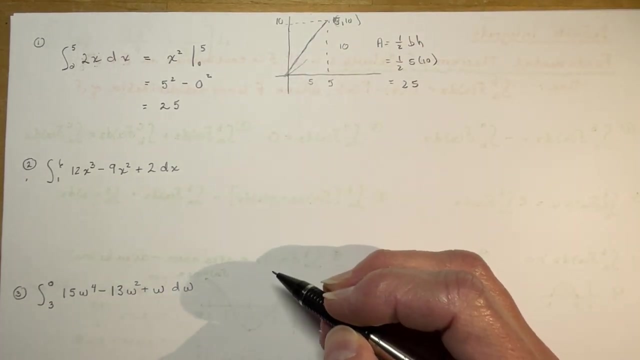 um, a height of ten. here I should probably have written this as five comma ten, so that gives me a height of ten and a length of five. so the area would be one half base times height, so a half of five times ten, and again that gives me 25.. So, um, if you've been doing Raymond sums and making all those 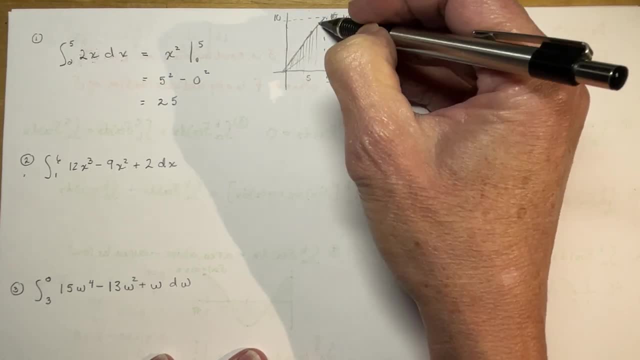 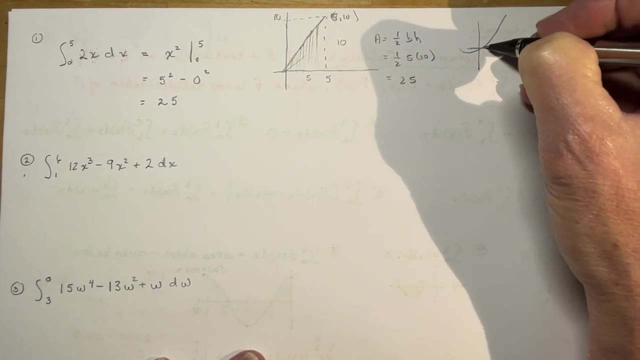 little triangles, remember. you make the triangle smaller and smaller and smaller, Especially on something like a curve. so if I wanted to find the area between the curve and the x-axis here, you probably started by making all these little tiny triangles. well, they're not triangles, they're um, what do you call those things? 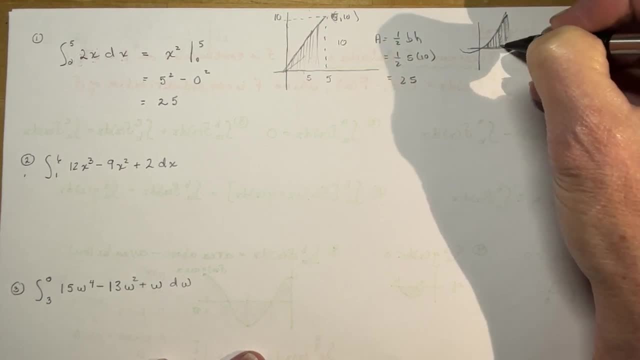 not rectangles- I can't think of the name right now, but I know you do, because if you've done Raymond sums, you've already added all these together and approximated the area, and then it's just like when you had to do derivatives from first principles. you learn all the hard. 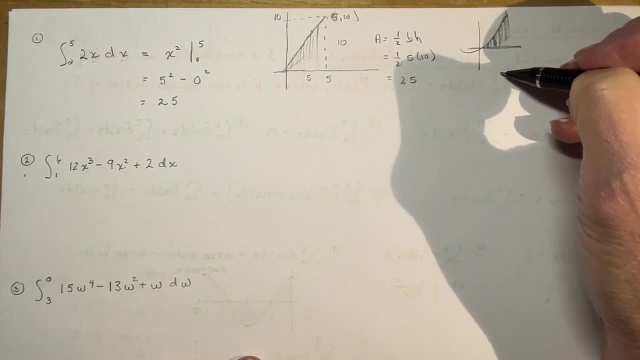 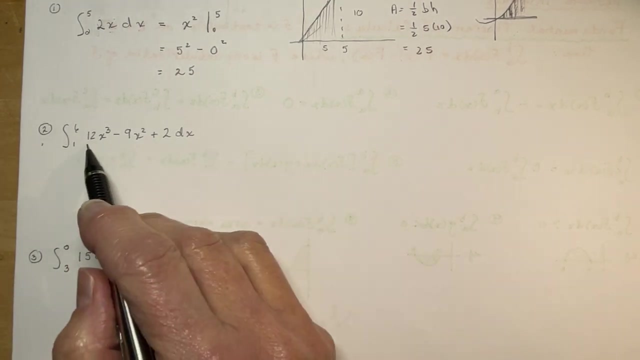 stuff and then say: oh, by the way, there are rules and you can find the derivative very easily. So instead of doing Raymond sums, you're going to be doing definite integrals. Okay, so let's try this one here. another pretty simple one. it's a nice polynomial. 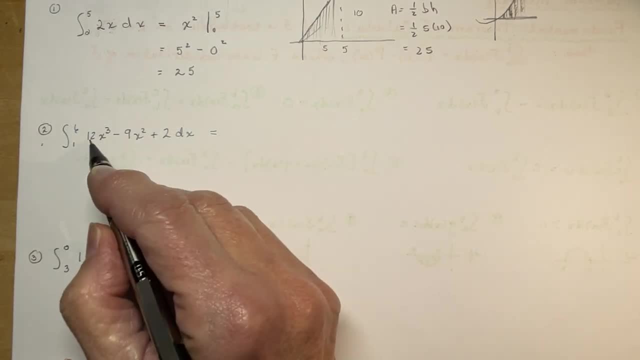 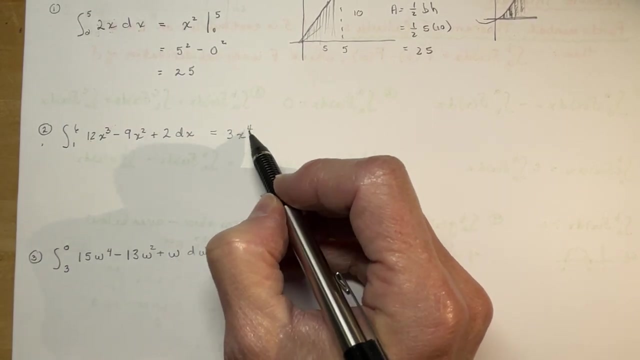 between one and six. so I'm going to take the antiderivative of 12x cubed. remember to add one and divide by that number, so three plus one is four. twelve divided by four is three, so three x to the fourth. and again, remember you can double check. 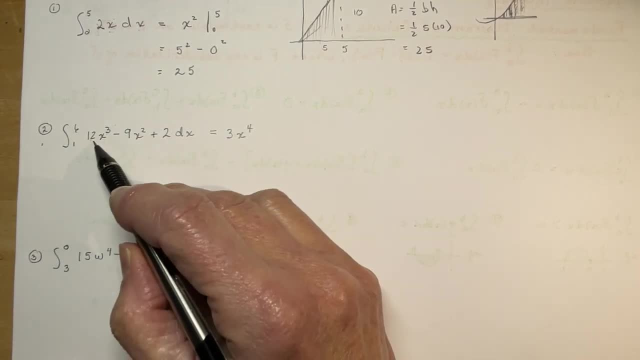 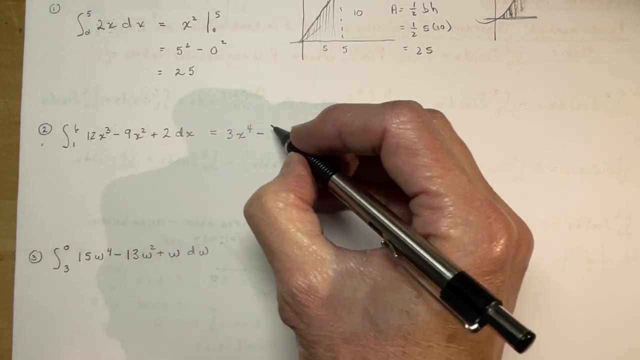 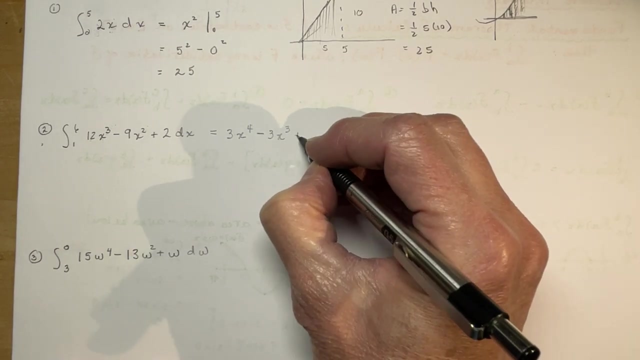 by doing four times three is twelve reduced by one and I get twelve x cubed. um, for the next one, I add: one makes three. nine divided by three is three and it is negative minus three x cubed. and this one is plus two and that's pretty easy. I get two x and I'm evaluating it between one. 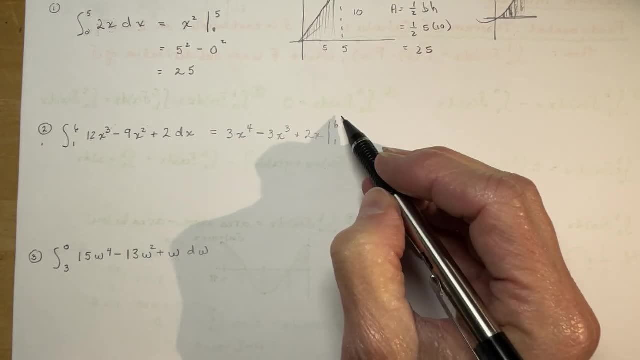 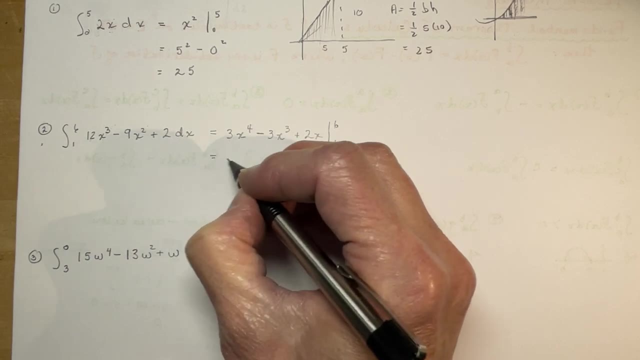 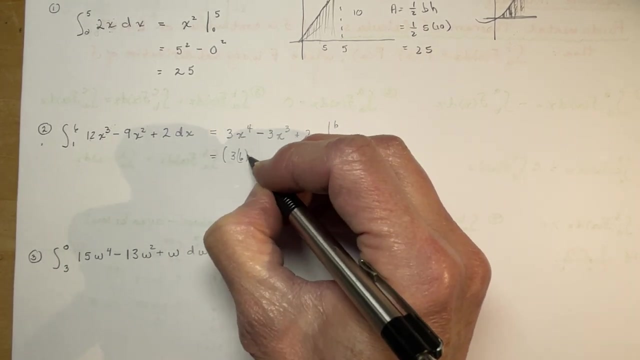 and six. remember that you don't need the plus c because we would be subtracting it away here. okay, so now it's just a matter of plugging in all your values, so I'm going to make a bracket here just to make sure that you keep all this nice and neat. three x to the fourth. 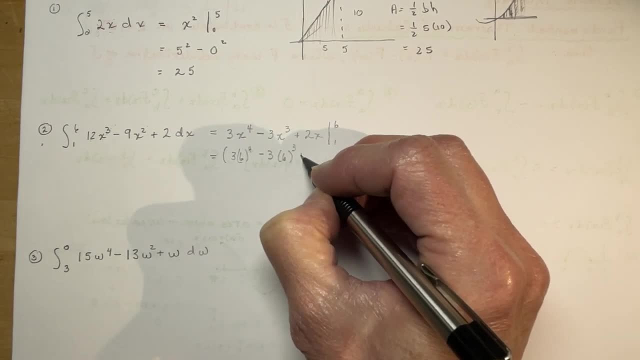 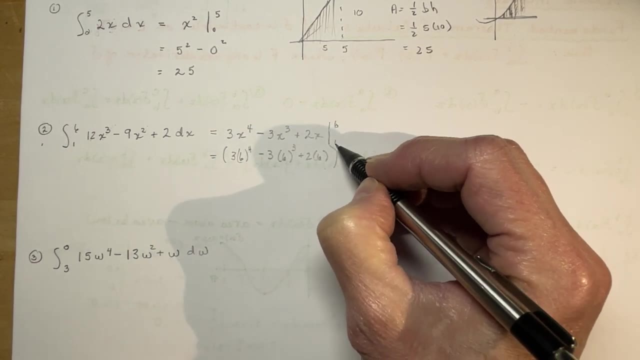 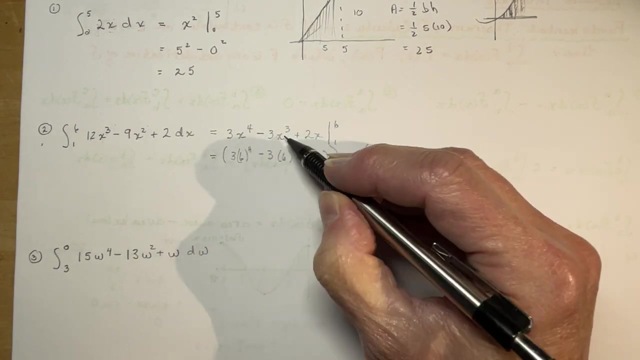 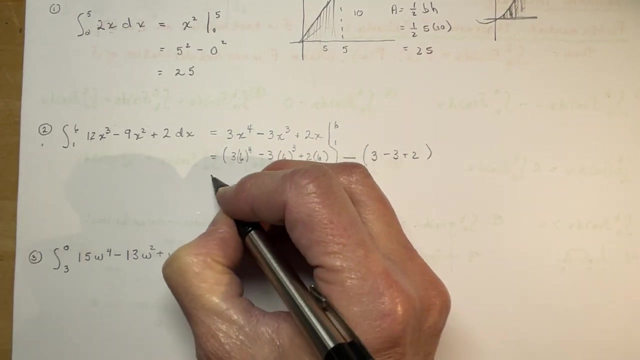 three times six, cubed plus two times six, and from that I'm going to subtract, so that's f at b minus f at a. so I'm going to subtract three times one to the power four is just three. and remember, if I'm plugging in one, everything becomes one. so minus three plus two, this one's. 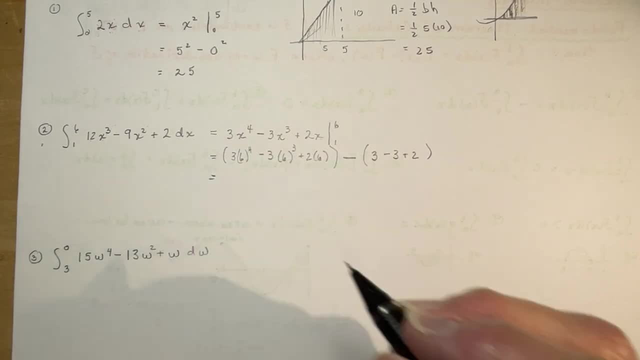 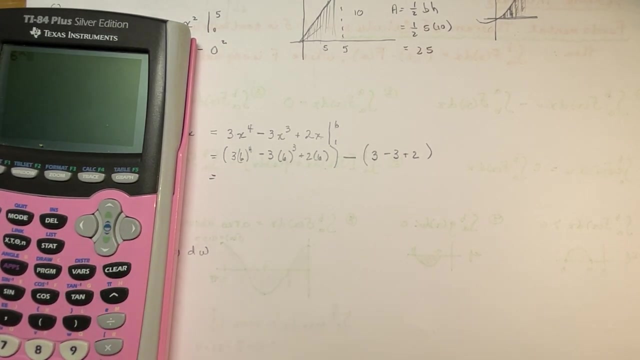 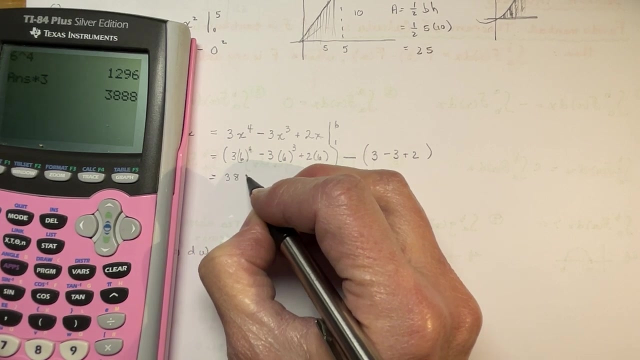 a little bit harder. you probably have to get out a calculator. six to the power, four. there's my calculator here. let's go find it hiding. it's hiding, but we'll bring it out. there we go, okay. so I'm going to do six to the power four times three. so I'm gonna write all these out for you. so three, eight. 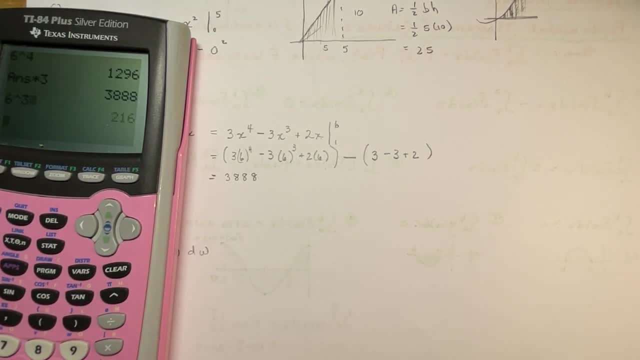 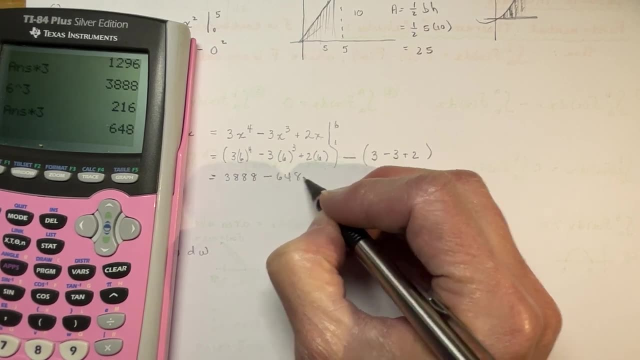 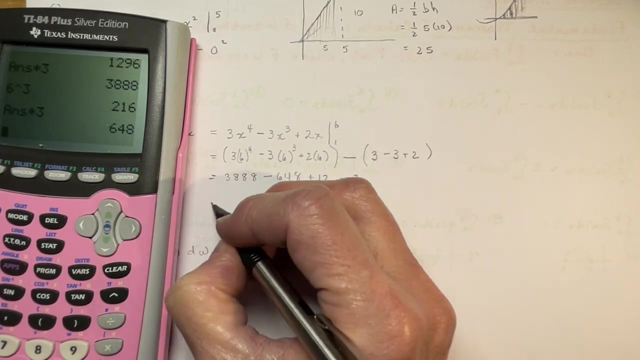 eight, eight, six to the power of three is two, sixteen times three is minus six. forty eight plus twelve and two, four plus six times three is six, and I'm going to count it out and I'm going to: and 3 minus 3 is 0, plus 2 is 2, and subtract 2, and if you do all that, I'm just going to tell. 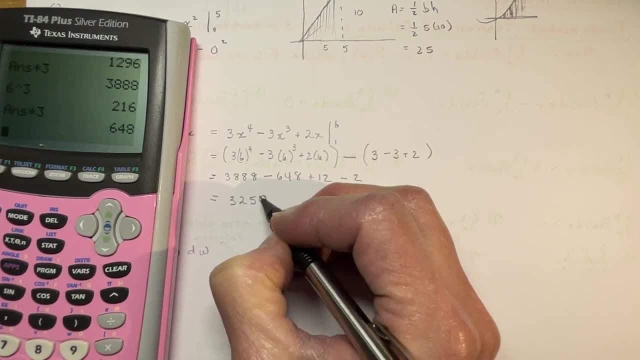 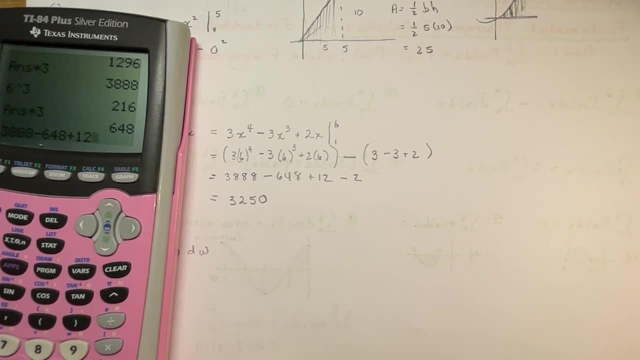 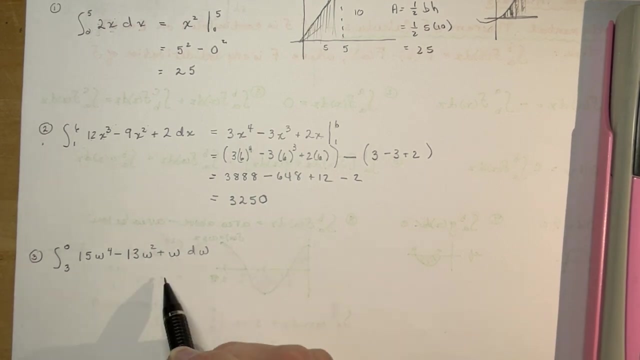 you what I got? I got 3250.. All right, we'll just double check it because I might have made a mistake: 648 plus 12 minus 2, and you'll get 3250.. Okay, so the next one here. notice it's from 3 to. 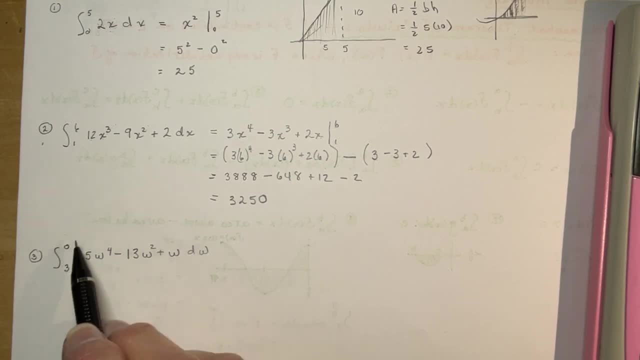 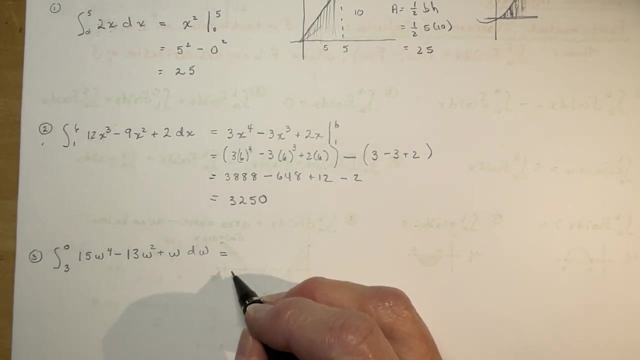 0, so you probably would guess that your answer should be negative. Sometimes it's a good idea to go on to Desmos and plot this so you can see and approximate to see. if it's the same as you might have guessed, it might be Okay. so let's do the antiderivative of these terms: I add 1 and divide. 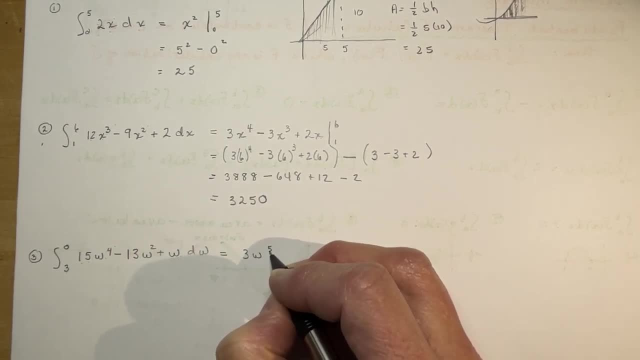 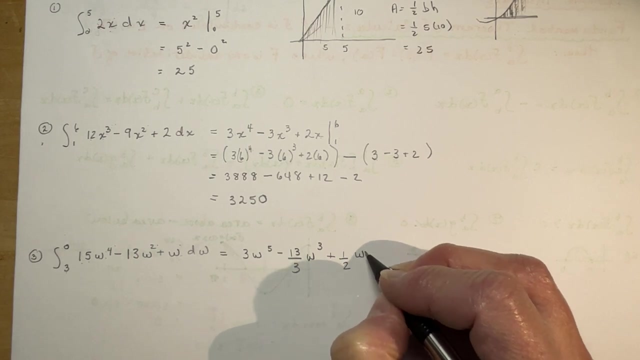 by 5.. That gives me 3w to the 5.. Add 1 is 3, minus 13.. Divided by 3w, cubed and I add 1.. That gives me 2. divided by 2 is a half w squared and that's. 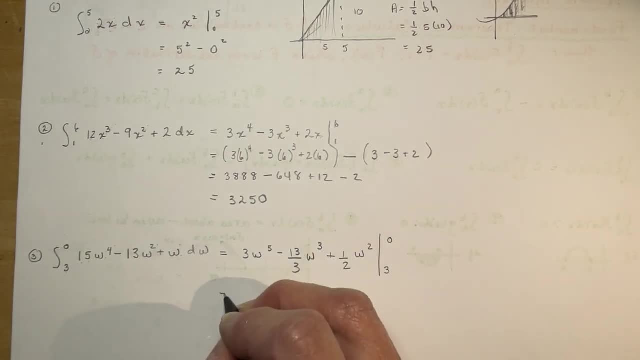 being evaluated between 3 and 0. So I plug in the 0 first. I always start at the top, so 0, 0, 0.. That was pretty easy and I'm going to subtract. Now I plug in 3, so it's 3 times 3 to the power. 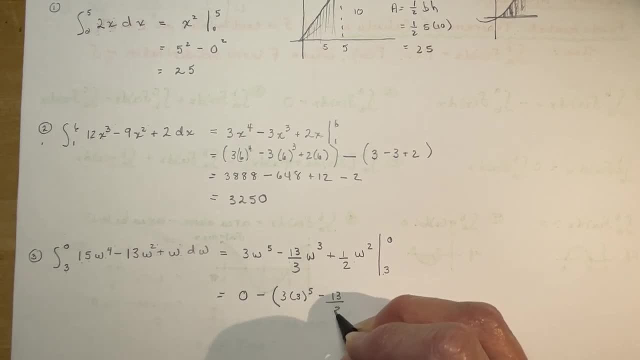 5.. Minus 13 over 3 times 3 cubed plus a half times 3 squared, So that's going to be 0, 3.. This is like 3 to the power of 6.. I'll do that quickly over on the side here and I get 729.. So I'm going to put. 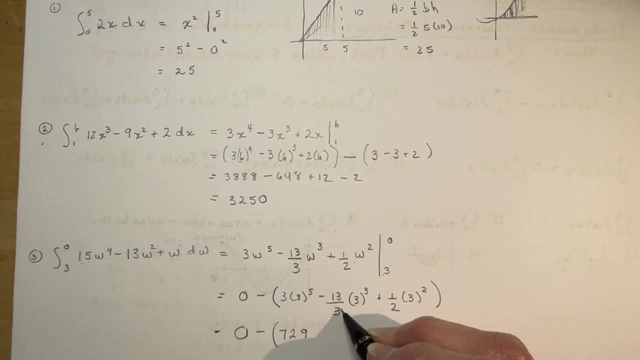 it in brackets, so I don't make a mistake. 3,. well, one of these 3s would make this a 2.. That's 9, and 13 times 9 is 117,. I think I'm going to double check that, because sometimes 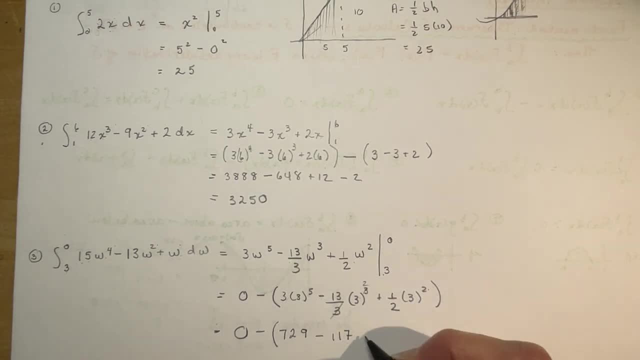 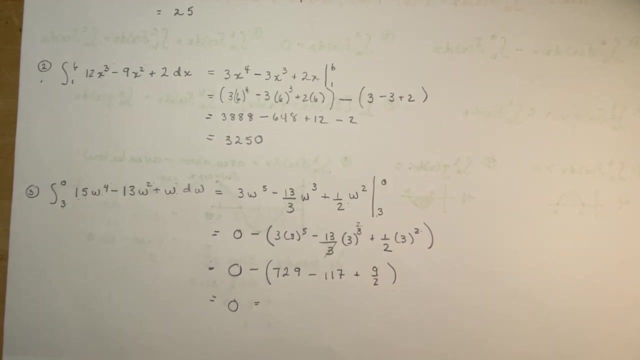 it's 117.. And this one, 3 squared, is 9, so plus 9 halves. So in order for you to get a nice answer here, you're going to have to put everything over 2, right, You need a half. So 729, 729 times 2. 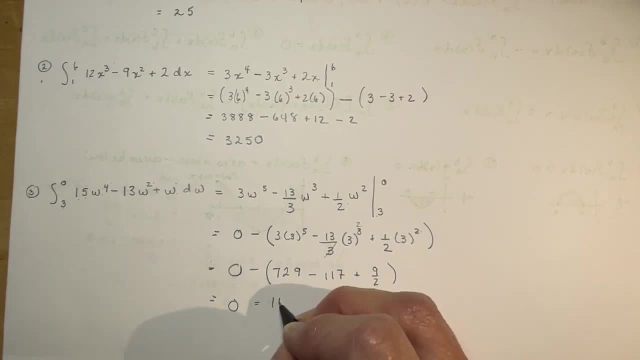 is 1450.. So that's 9,, and 13 times 9 is 117.. So that's 9,, and 13 times 9 is 117. So that's 9, and 1458.. I don't know why I put that. That's a minus 1458,. this is all going to be over 2.. 117. 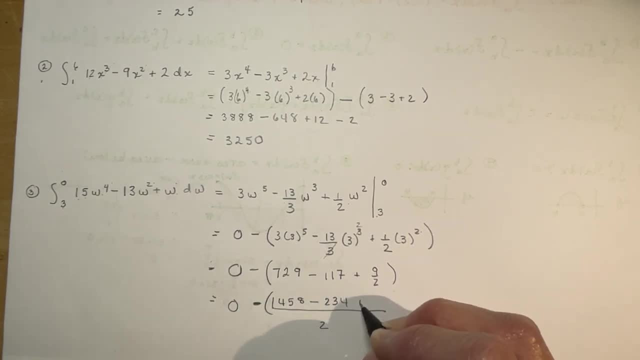 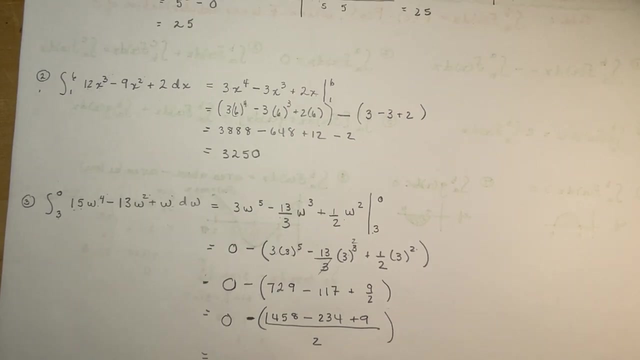 would be minus 234, plus 9,, all over 2.. And you should get negative 1233 over 2.. And there you have it. It's not all that hard, is it? Okay? but of course you're going to have to put everything over 2, right? So you're going to have 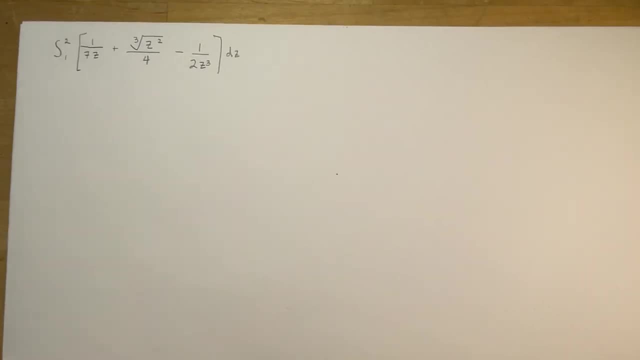 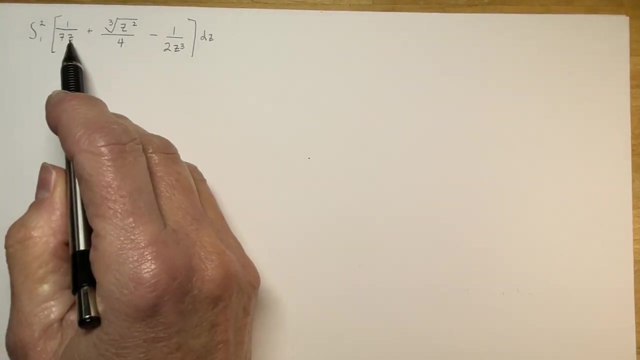 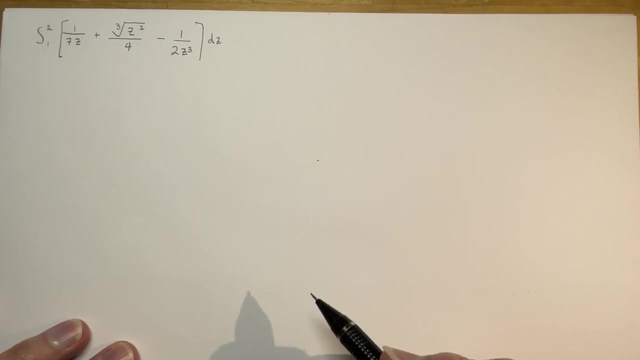 some of the definite integrals have trickier little things in them, like this one here. So the first thing I would suggest- and these are zeds here- I put a line to them. They're not twos with lines or anything like that. So the first thing I'm going to want to do is 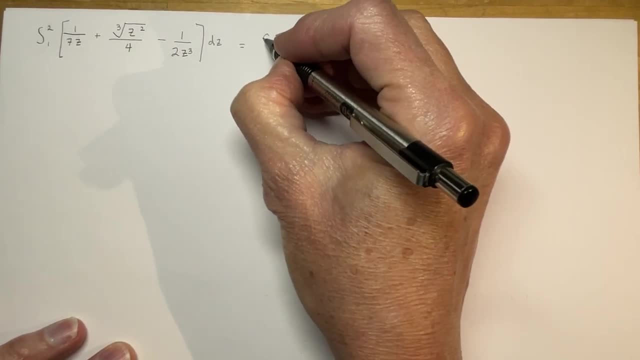 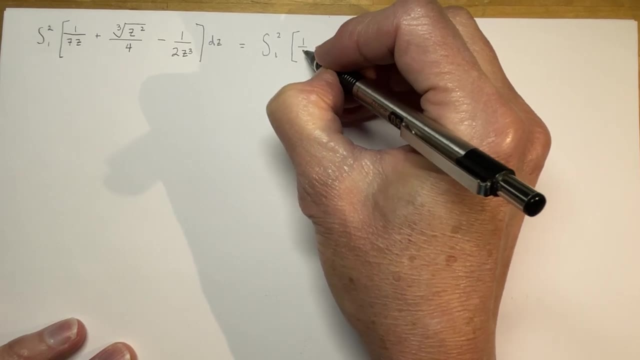 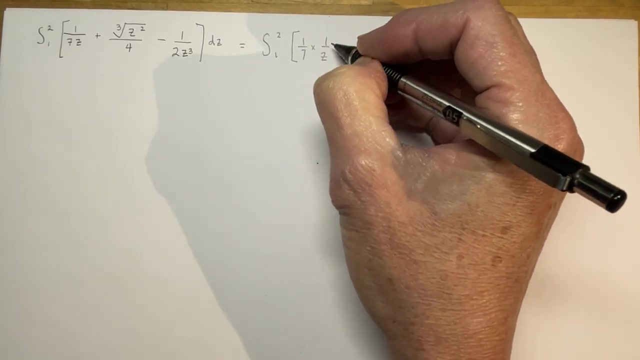 make this just a little bit easier to understand, right, I'm going to write it as the integral between 1 and 2 of put a bracket. So I'm going to take the 7 out 1 7th times 1 over zed, because I know the antiderivative of 1 over zed is the law of zed. 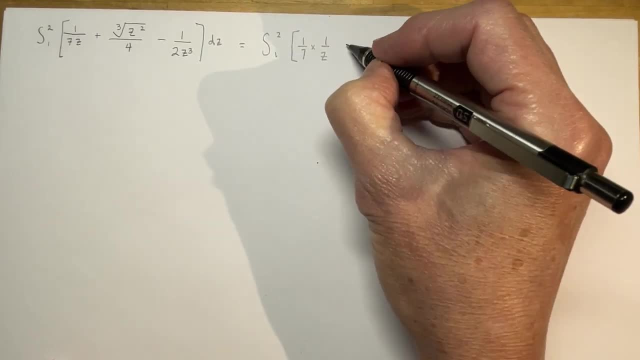 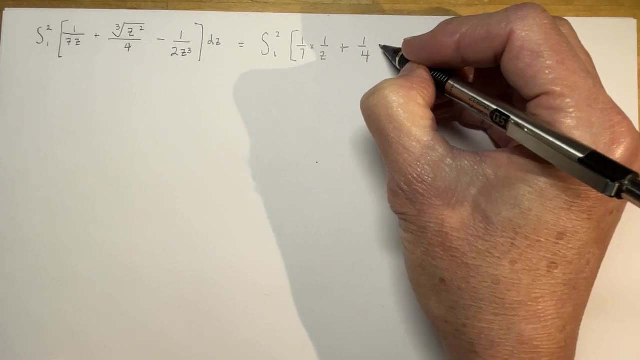 right, I'm not going to put it to the numerator, not that one, And I'm adding. so this is 4 in the denominator. So let's kind of make this a quarter and it's going to be zed to the power. remember: this is the exponent, This is your. 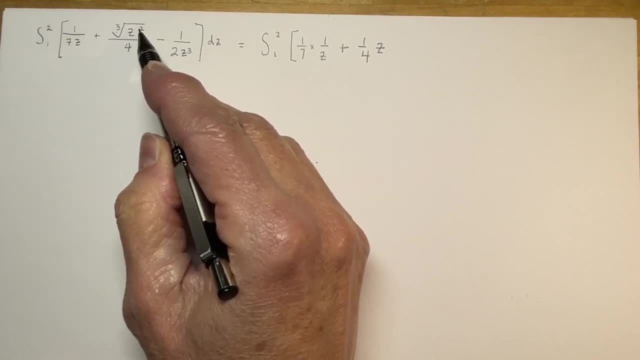 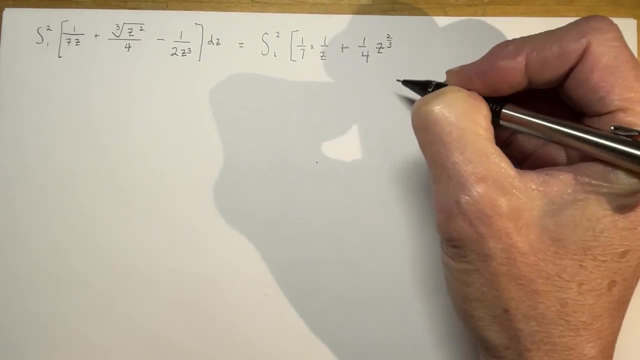 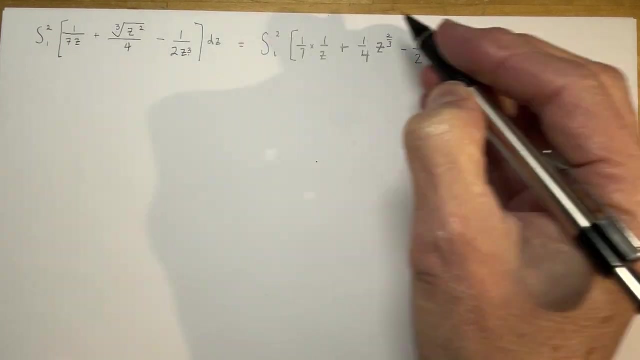 um, sort of the part, the top of your numerator, your fraction. This is the bottom, So it's two thirds power- It'll be easier to work with, And minus one half, and the zed is in the denominator. I bring it to the numerator. That makes it negative. 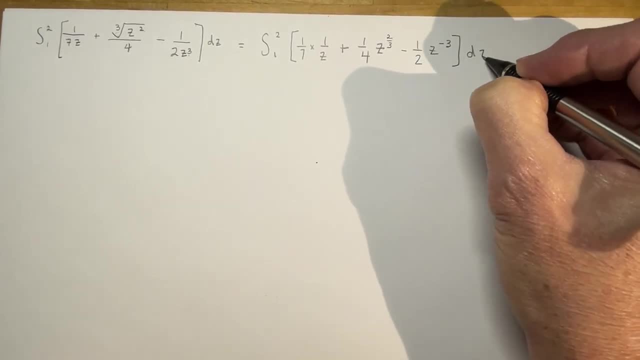 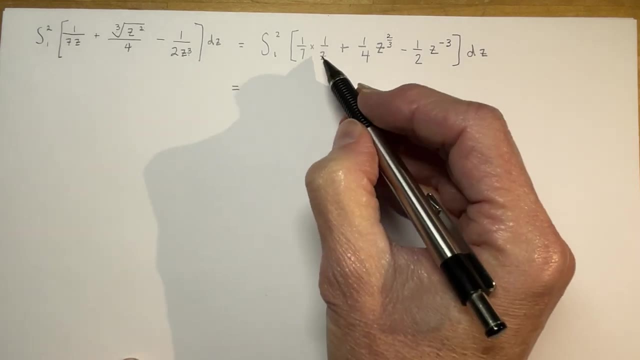 Okay, so I hope I'm not making you sound like this is all. I'm over explaining things, but sometimes you just forget things, right? Okay? so I want to take the antiderivative here, So this is going to be 1,. 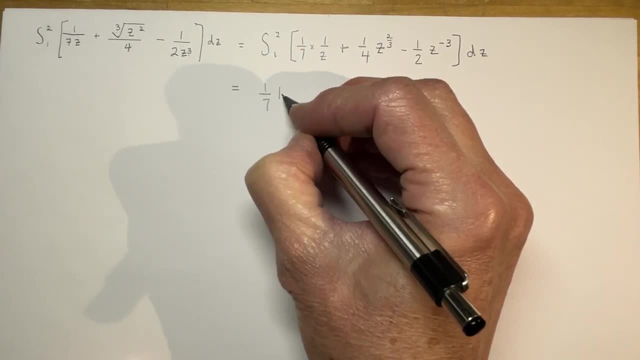 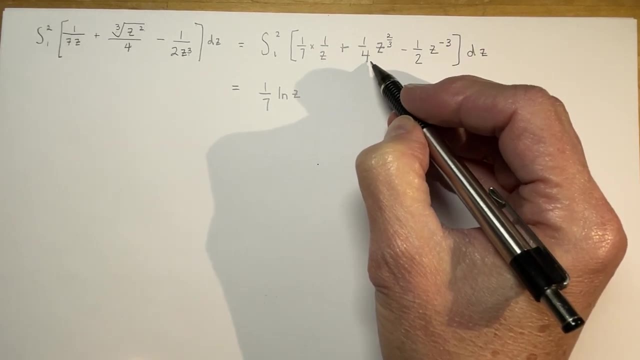 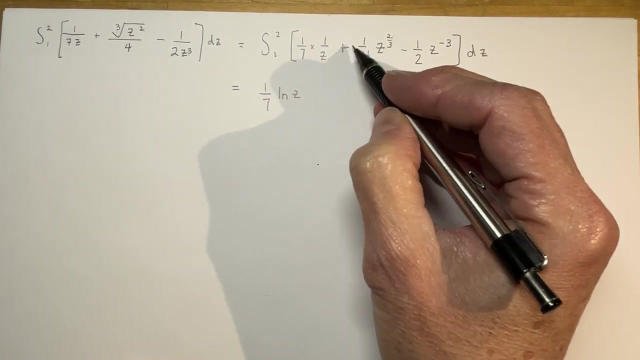 over 7, and 1 over zed is going to be the lawn of zed, lawn of zed, And this 1 over 4, I add one to this, So that's going to make it 5 over 3.. I'm going to multiply by 3 over 5.. 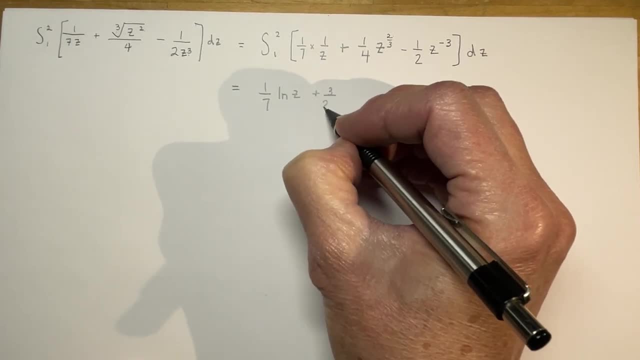 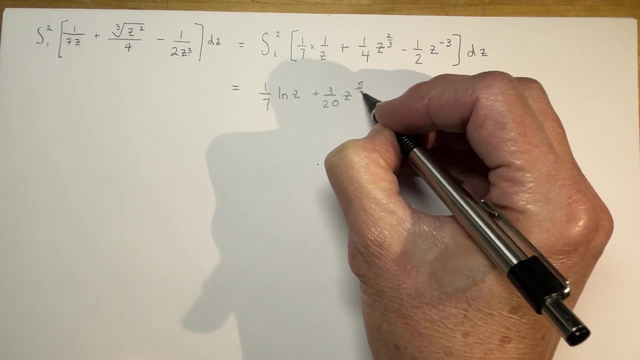 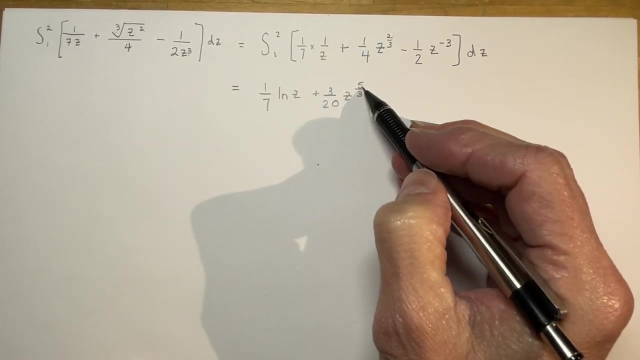 That's going to give me plus 3 over 20 zed to the uh, add 3.. So to the 5 over 3, now you can see quickly if I multiplied this by this by taking the derivative to check my answer. 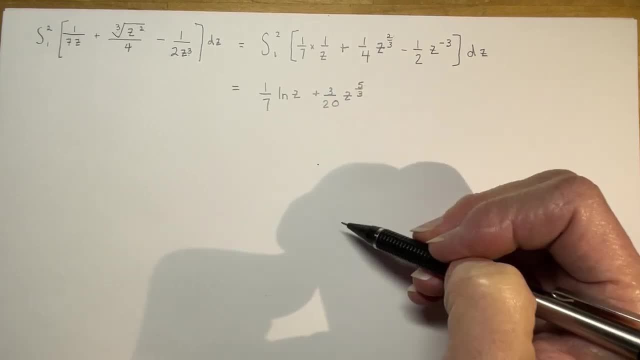 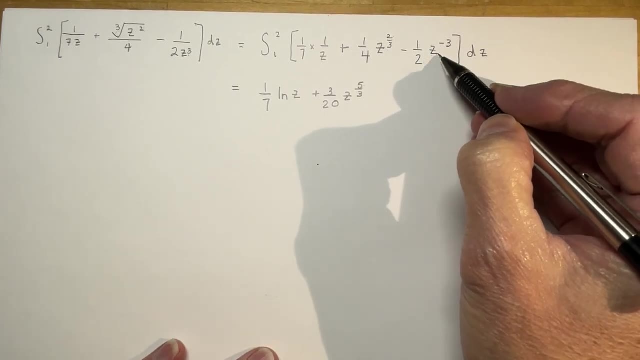 uh, 5 will go into 24 times and those 3s would cancel out. And the last one: here I'm going to add 1 to minus 3.. Don't forget: when you add to a negative, it becomes less negative. So that's going to be minus 2.. 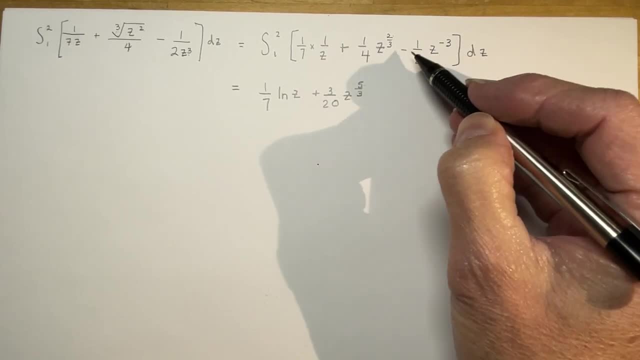 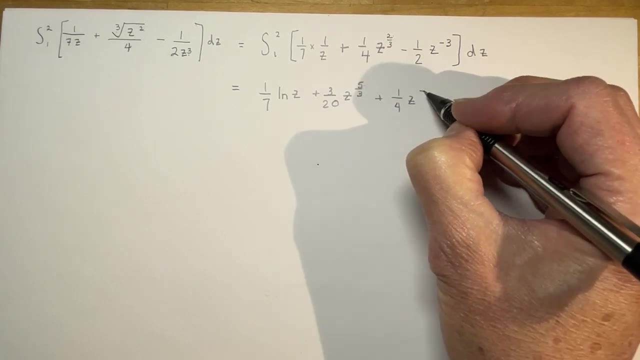 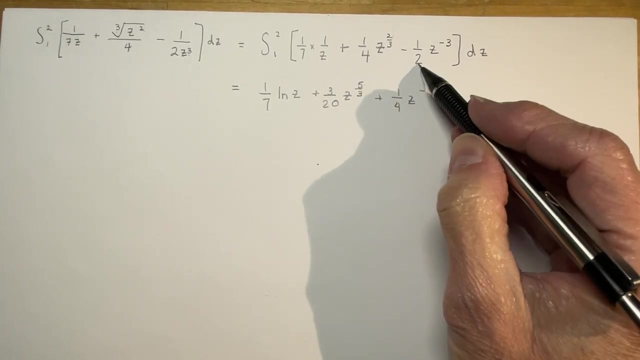 So I'm dividing by minus 2.. So that's going to give me a quarter here. Half times a half is a quarter Zed to the minus 2.. So again I would check, Minus 2 times this would be minus 2 quarters is a half. 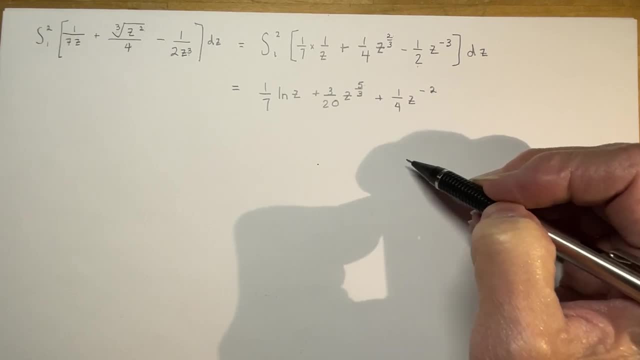 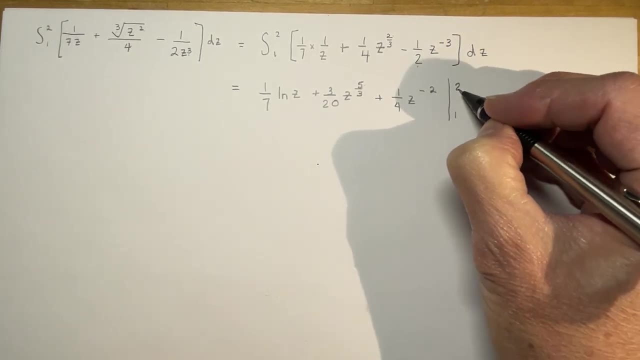 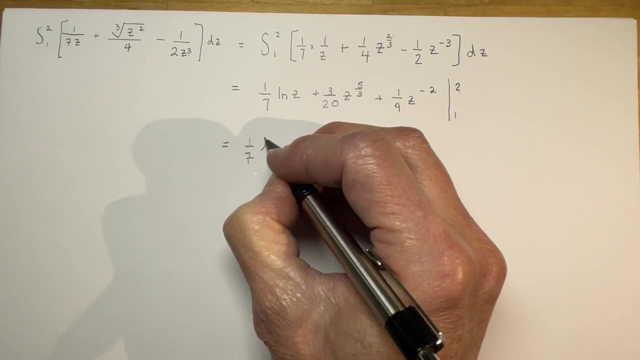 And reduce this by 1 would be to the negative 3.. And that whole thing is going to be evaluated between 1 and 2.. So now I have to plug in 2 first, So I have 1 over 7, lawn 2.. 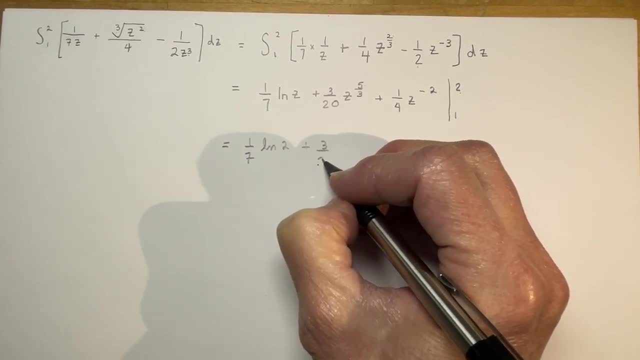 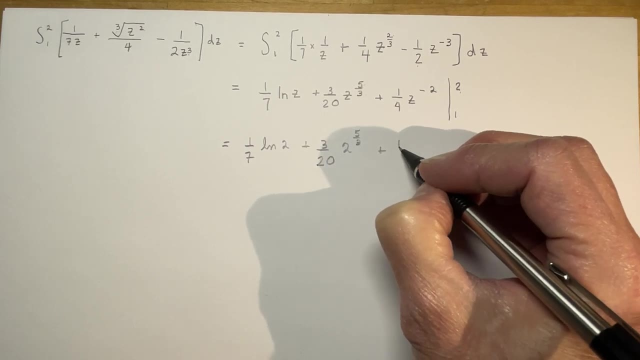 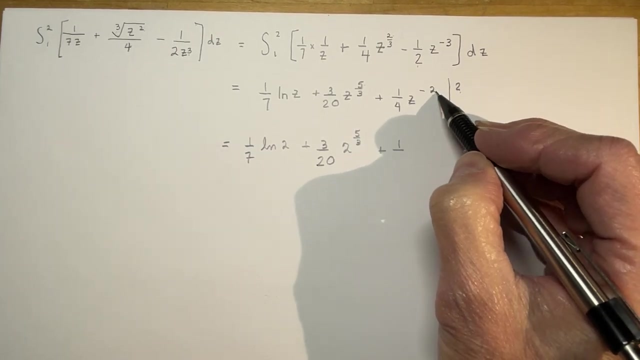 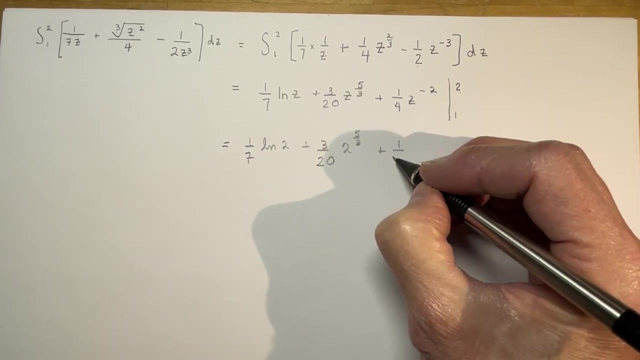 Plus 3 over 20 times 2 to the 5 thirds plus 1 over. okay, now we can fix this right at once. This is 2 to the negative, 2.. 2 to the negative 2 is 1 over 2 squared. That's 1 over 4 times 1 over 4.. 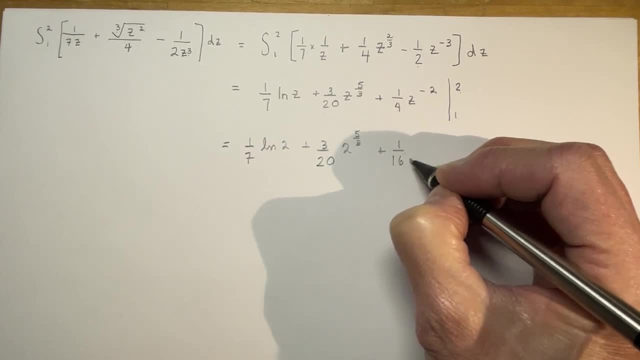 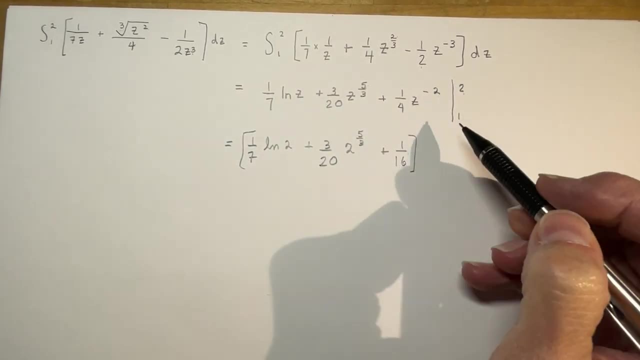 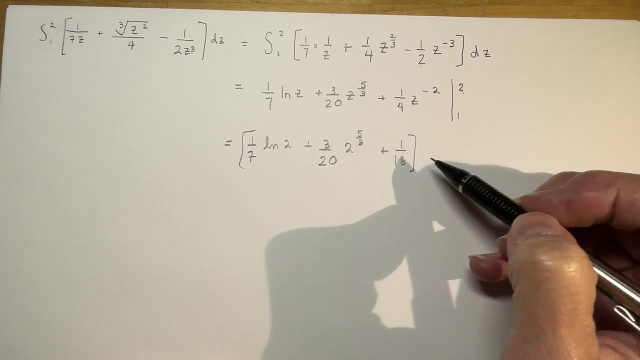 That's going to give me 1 over 16.. Okay, So that's just the first part, right? Remember that you have to make sure that you do this and then minus that one, right? So right now, I've got all this done and I'm going to subtract. 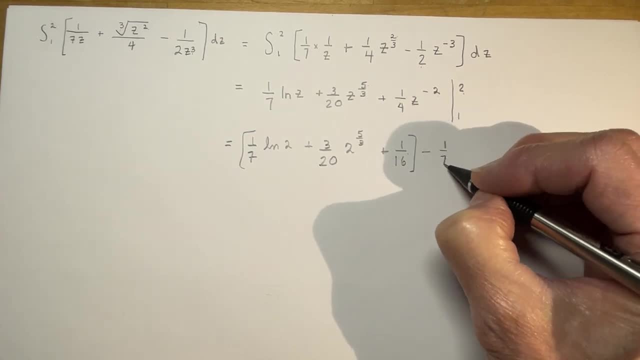 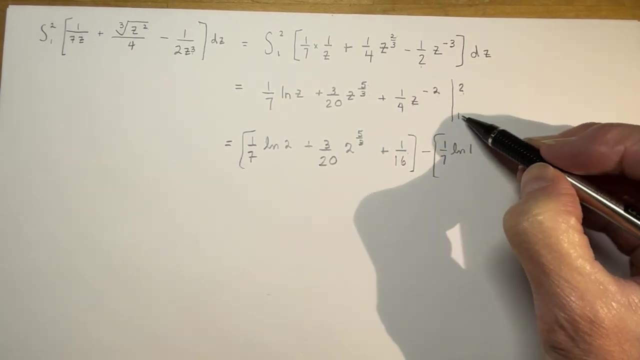 Subtract and I'm going to plug in 1.. So 1 over 7, lawn of 1.. What's a lawn of 1? I'll let you think about that for a minute while we finish this. I plug in 1 here. 1 to any power is 1.. 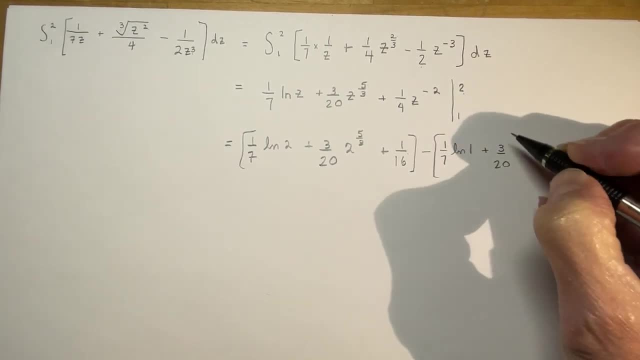 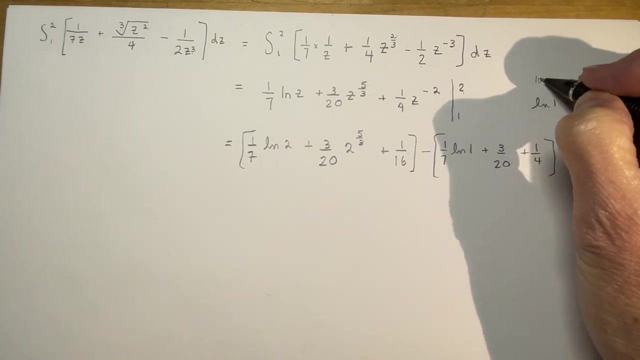 So I'm going to be adding 3 over 20.. And 1 here is just going to be 1 quarter. So do you remember what the lawn of 1 is equal to? Lawn 1 equals. in other words, if this would be if you wrote that as log base e of 1,. 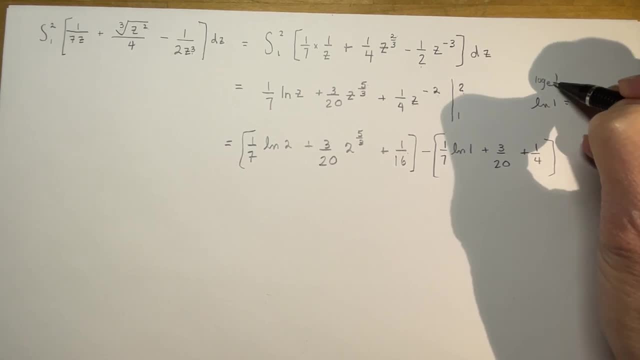 I'd say: what do I raise e to? What power do I raise e to? to get 1?? And your answer is 0.. Okay, so that's going to be 0. And 3 20ths plus 1 quarter, that would make 8 20ths. 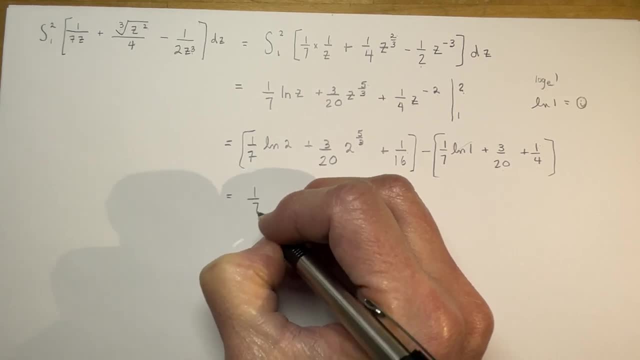 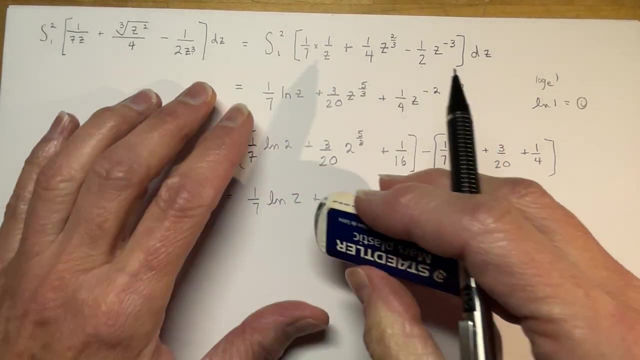 So we have a little bit of fraction work left here to do So. just a minute. that looked like I wrote it as a z. It's supposed to be a 2. It's probable when you work with z's and numbers, right. 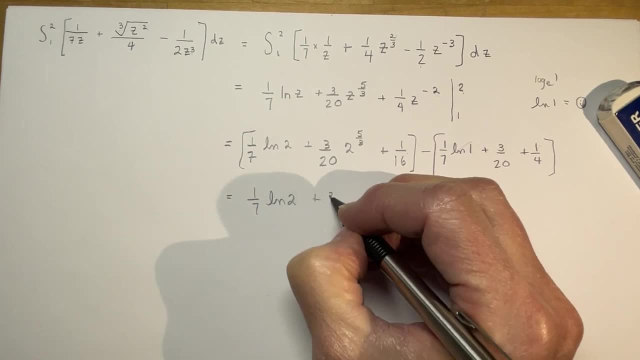 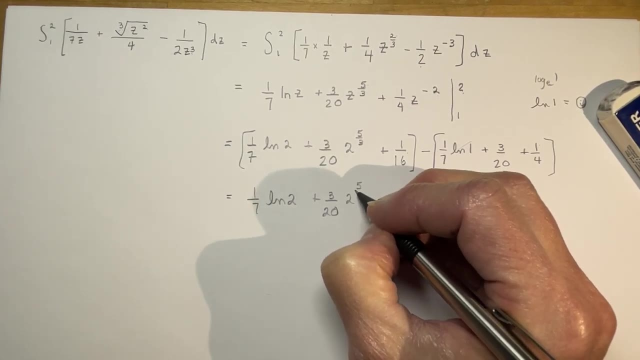 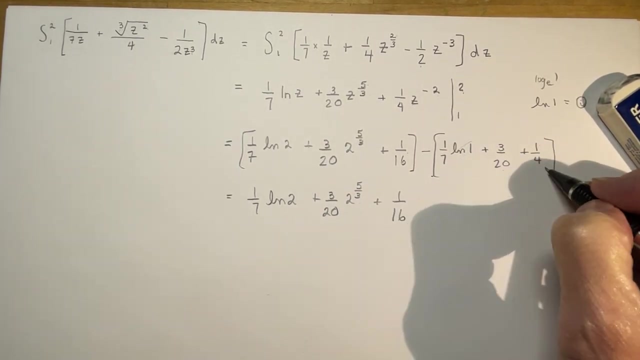 Lawn: 2 plus this- I don't know what- the third root of 2 is raised to the fifth power, So I'm just going to leave it as 2 to the 5 thirds Plus 1 over 16.. And this we had said this was going to be 8 over 20.. 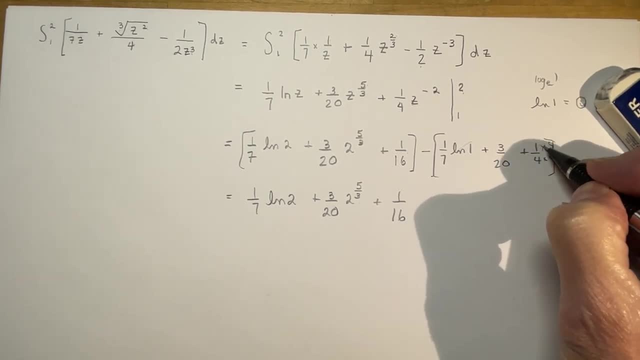 Because this is times 5 times 5. And 5 plus 3 is 8. Plus 8 over 20.. So the only part I'm going to just work with is this: What is the lowest common denominator of 16 and 20?? 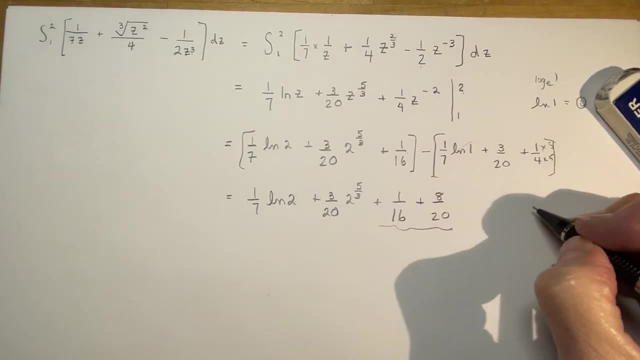 That would be 80. So 16 is 5 over 80.. 1 over 16 equals 5 over 80. And 8 over 20 is the same. 8 over 20 is 32 over 80.. Okay, so that's just on the side here. 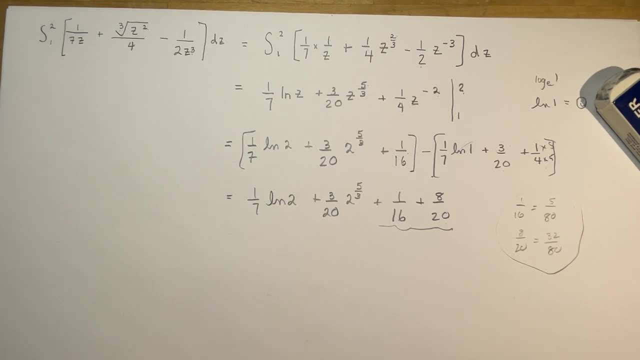 So I'm going to add those two together to get Just a minute. I forgot a bracket here, didn't I? Oh, Ms Havron, They should have been subtracting this 8 over 20.. Because this was positive. 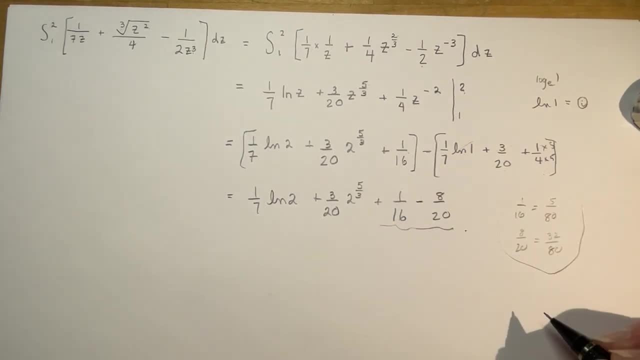 8 over 20 and minus it. So it should have been minus 8 over 20.. So I have 5 over 80 minus 32 over 80. That's minus 27 over 80. And the rest of this. 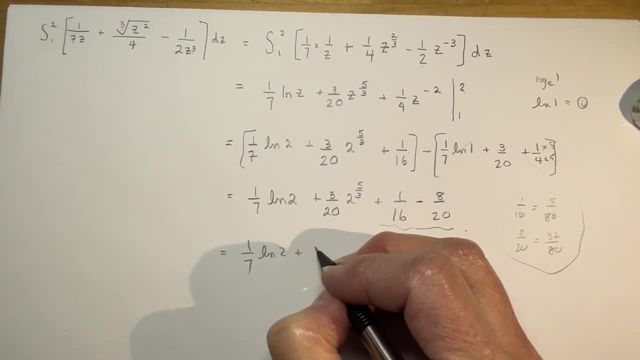 And that's the way I'm going to leave my answer, Unless your teacher asks you to write it as a decimal, In which case you would get out your trusty calculator And, you know like find the cube root of 2.. 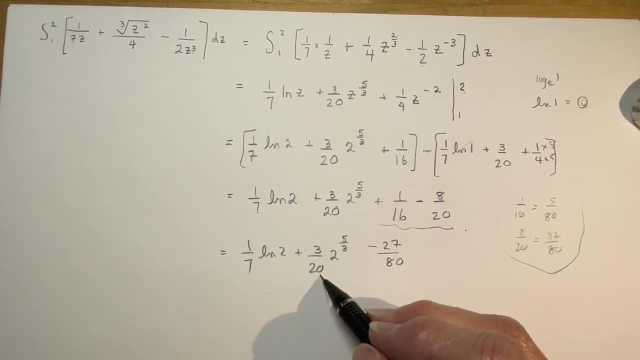 Raise it to the power 5.. Multiply by 3. Divide by 20. for that one You can find the ln of 2 easily. Divide it by 7. And you can make this into a decimal as well. Okay, so that's a little introduction to definite integrals. 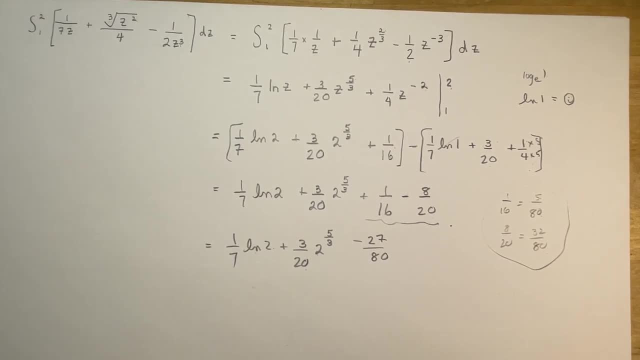 If there's something more specific you need help with, just let me know. Don't forget to subscribe, like, comment, share And yeah, have a great day. 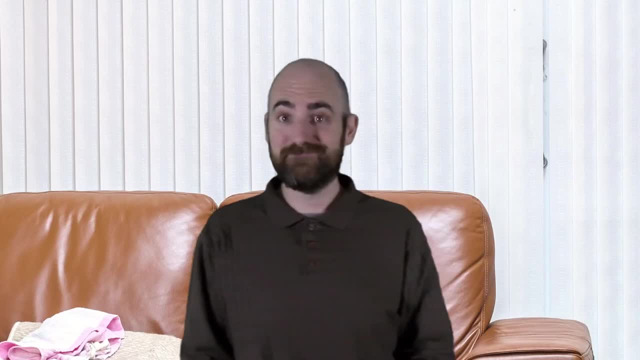 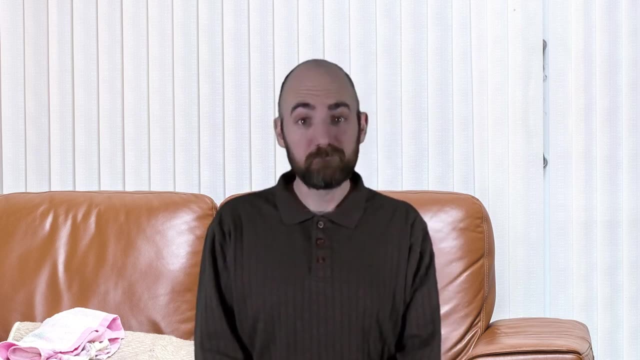 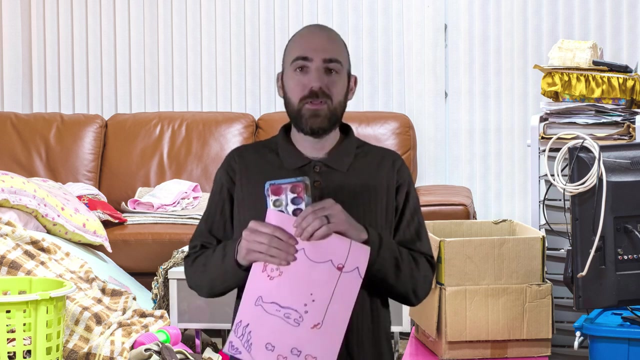 Hello friends, we'd like to introduce you to a very special person today. This is Jesse. Jesse is just like you. He lives in a house and he is good at a lot of things. He especially likes arts and crafts. Hmm, it looks like he made a little bit of a mess. 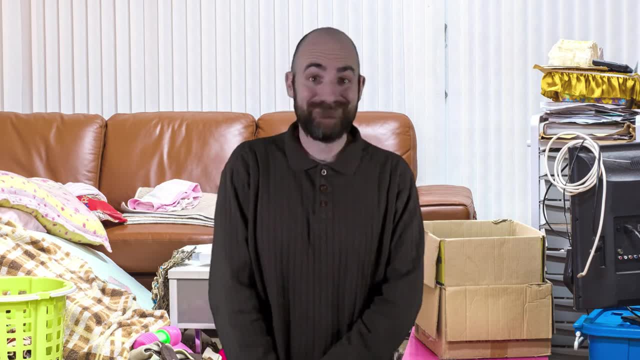 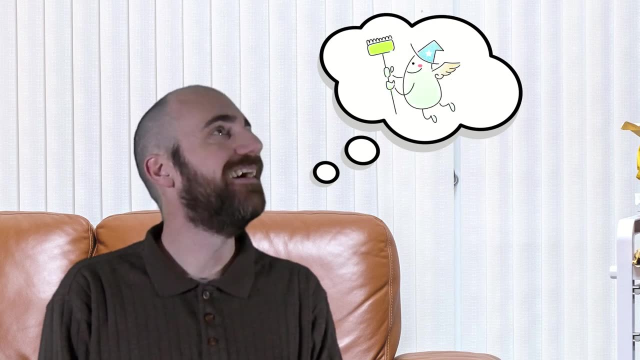 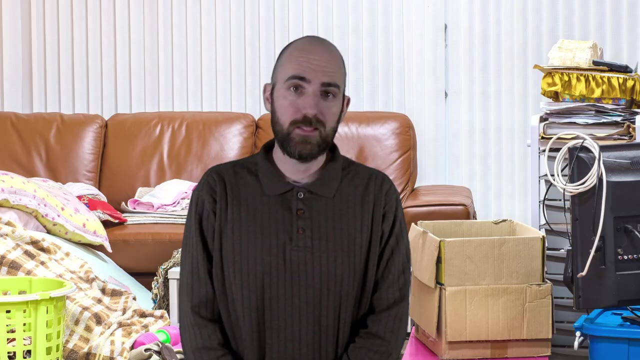 Yes, he's good at that too. Jesse doesn't like cleaning up his messes. In fact, his whole life he always thought there was a magical cleaning fairy who did that. Sadly, there is no magical cleaning fairy. Jesse has just always had other people around who cleaned up for him.